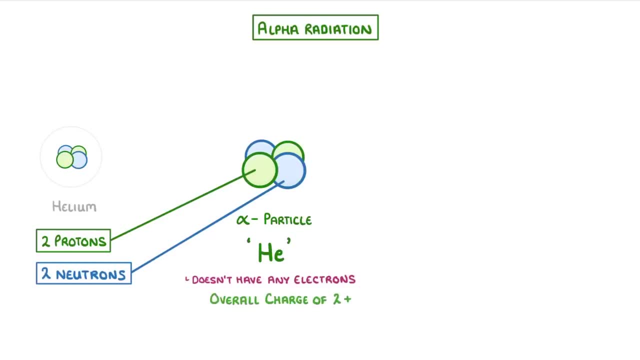 charge of 2+ from those two positive protons. Because they are relatively large, alpha particles are easily stopped by collisions with other molecules, which means that they can't penetrate very far into other materials. In fact, they can only travel a few centimetres in the air and are absorbed by a single sheet. 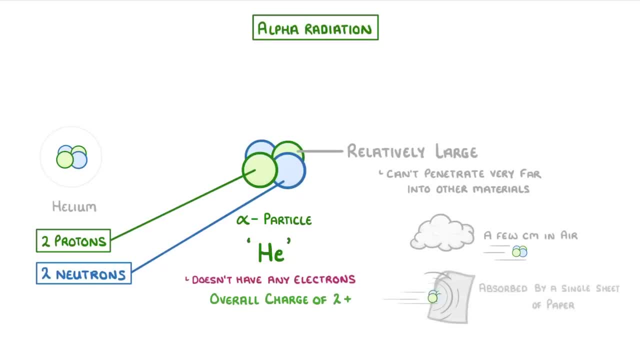 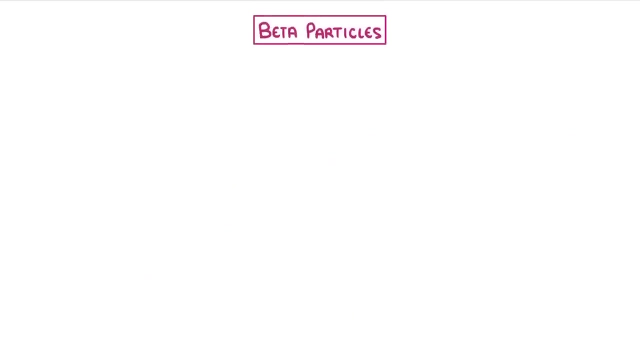 of paper. However, their large size and their strong charge does make them very strongly ionising, which just means that they can easily knock electrons off any atoms that they collide with. Next up, we have beta particles, which are just electrons, So they have a charge of minus one and virtually no mass. 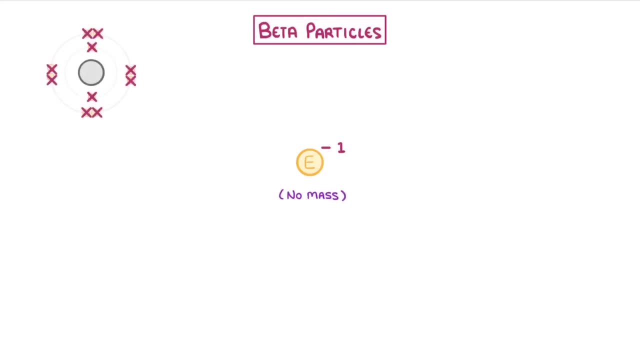 Now the weird thing is that electrons aren't emitted from one of the atom's shells. Instead, one of the atom's neutrons decays into a proton and an electron. The proton stays in the nucleus, but the electron is emitted out at high speed. 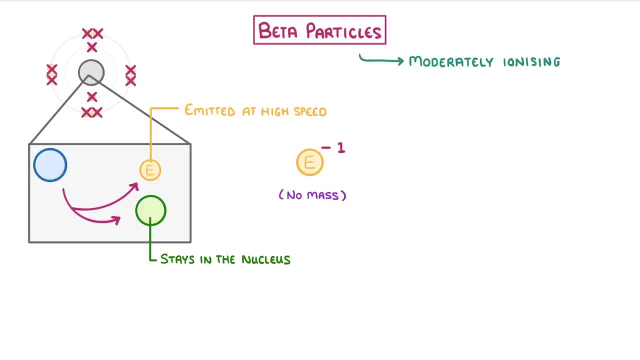 Because beta particles are pretty tiny, they are moderately ionising and they penetrate moderately far into materials. For example, it would take several metres of air or about 5mm of aluminium to stop them. Now, gamma rays aren't particles at all. 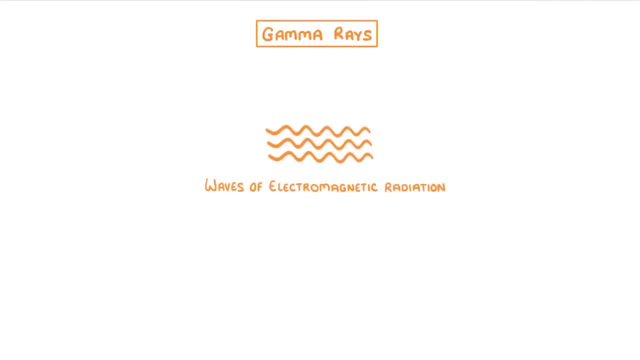 They're actually particles. They're actually waves of electromagnetic radiation like lighters, And they're often emitted after alpha or beta radiation as a way of the nucleus getting rid of a bit of extra energy. As they don't have any mass or charge, they tend to pass straight through materials rather. 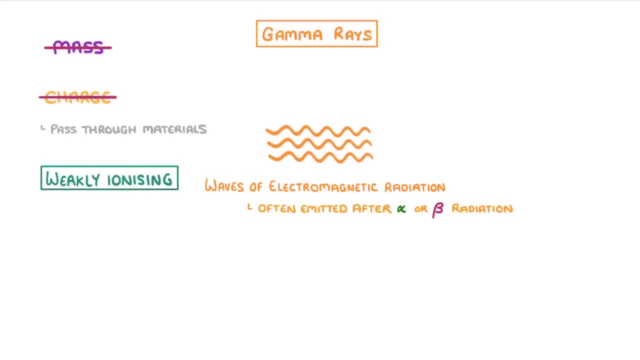 than colliding with any of the atoms, which makes them only weakly ionising. This means that they can penetrate really far into materials before being stopped. So it can travel long distances through air and it takes thick sheets of lead or multiple. 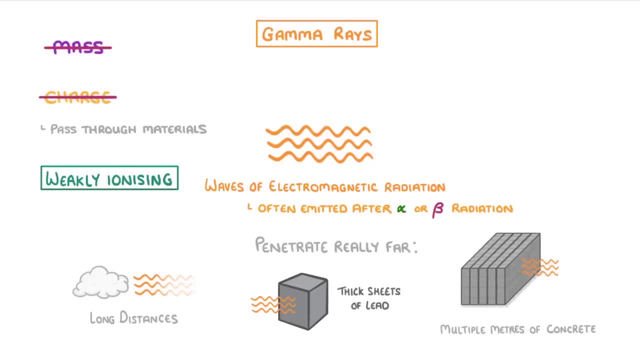 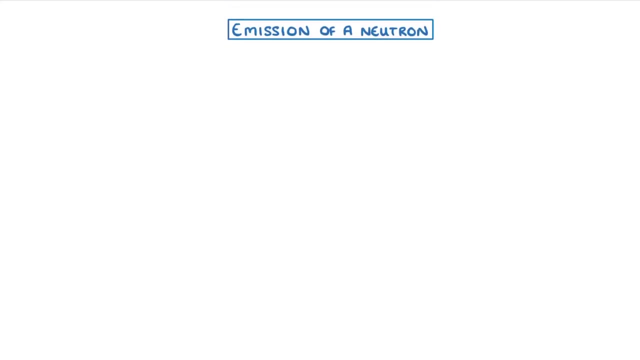 metres of concrete to stop them. The last type of radiation we need to look at is the emission of a neutron, And there really isn't much to know. If a nucleus contains too many neutrons, which is making it unstable, it can just throw out.